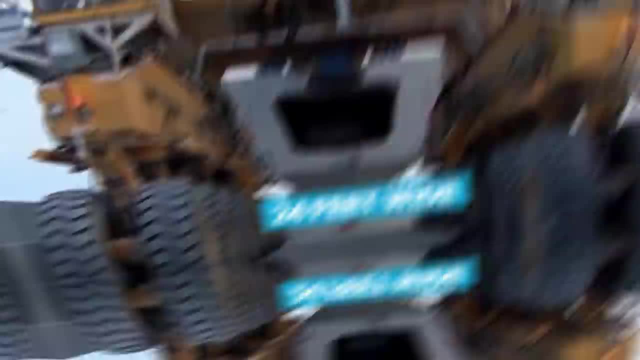 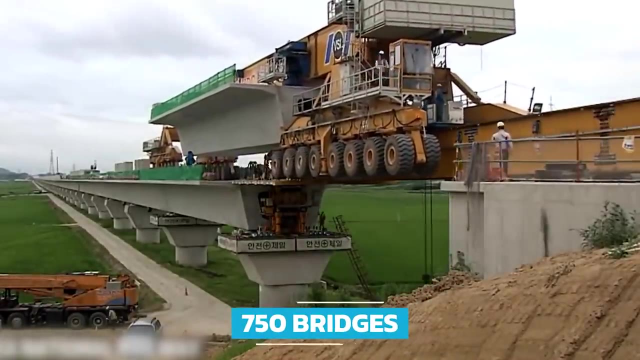 The SLJ-900 is almost 300 feet long, 24 feet wide and weighs a monstrous 580 tons. A single SLJ-900 can help create almost 750 bridges in its lifetime. The machine only needs the pylons of the bridge to be properly erected in their places. 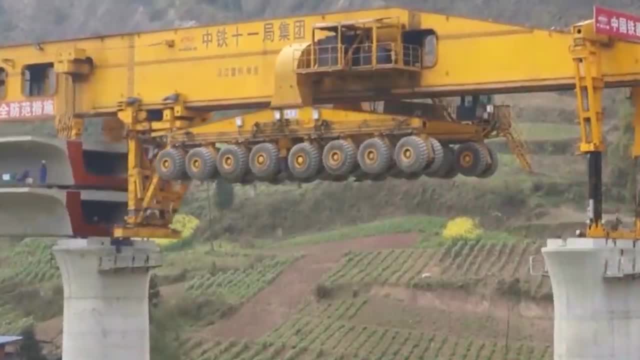 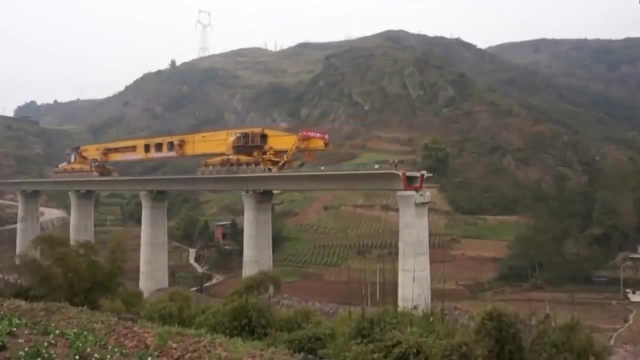 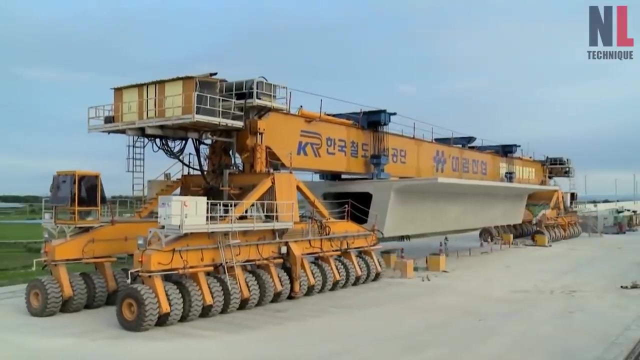 As long as the pylons are properly installed, the SLJ-900 can extend past the pre-made bridge segment to lay down a further segment. Once the segment has been laid down, it can go back and bring forth another segment to be laid down, Even while carrying maximum load. the SLJ-900,. 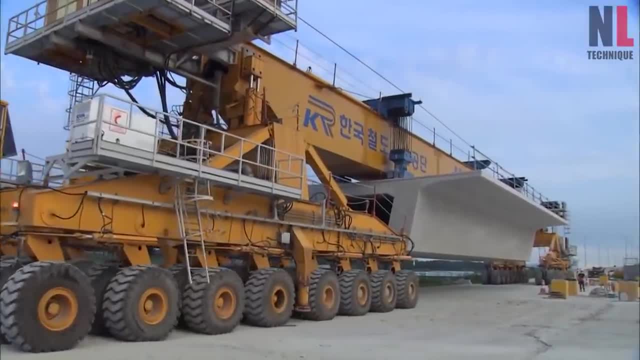 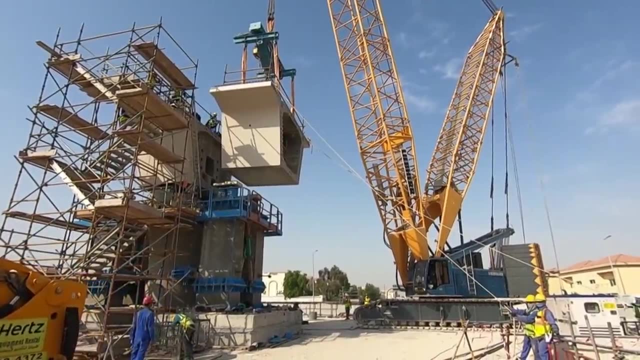 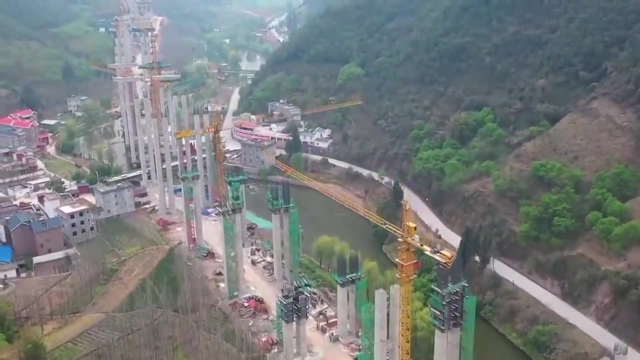 or the Iron Monster as it is commonly known, can move at almost 5 km per hour, which makes it light speeds- faster than a stationary crane that has to stay rooted on the spot to lay down bridge segments. Before the SLJ-900 was developed, bridge sections were laid down with the help of huge cranes. 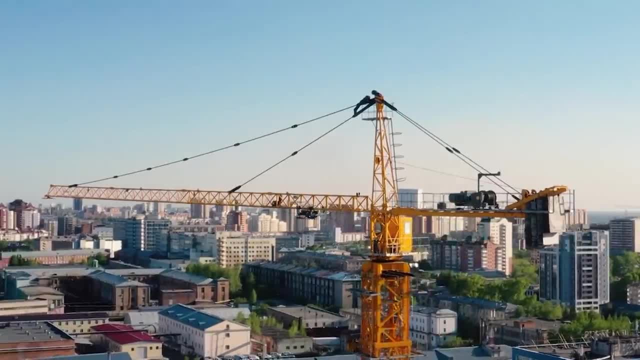 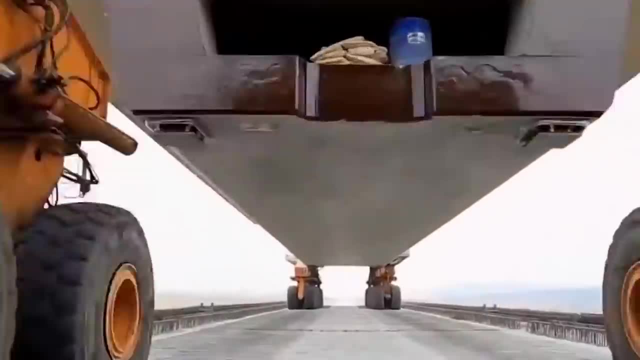 Anyone who has seen a crane work knows how painstakingly slow it can be to use a crane for construction. It not only requires time but also a lot of labor, whereas the Iron Monster only requires a minimal amount of labor, thus reducing the overall cost of the project. It can roll on its 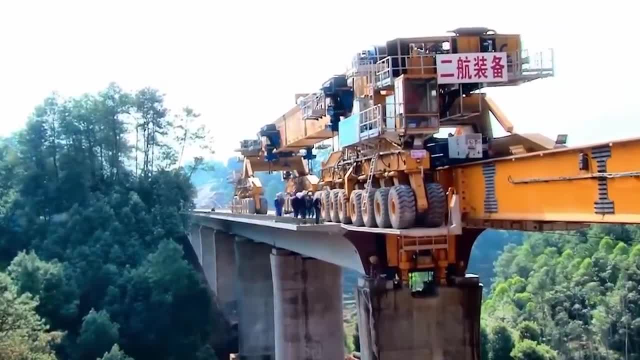 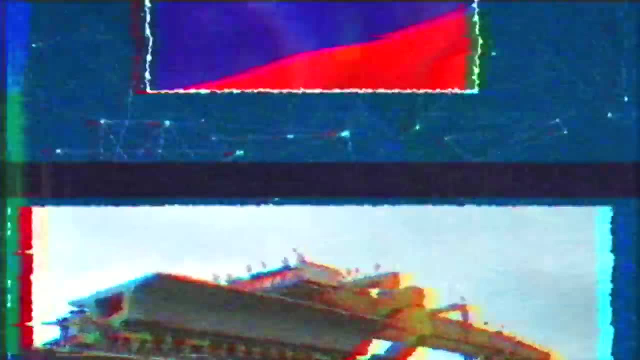 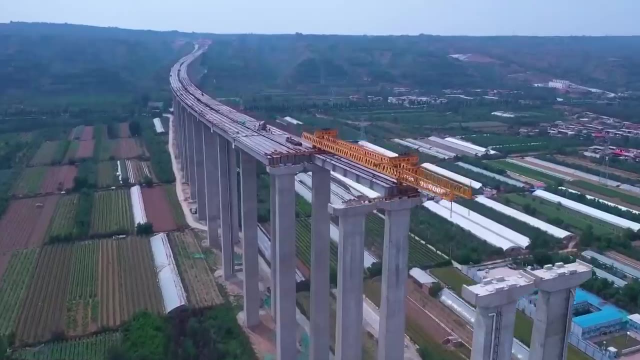 64 wheels, both forward and sideways, carrying bridge segments and laying them down. The SLJ-900 is a groundbreaking development in the world of bridge construction. Countries like Russia and India are already eyeing to purchase it from China. It can be particularly helpful in building bridges over 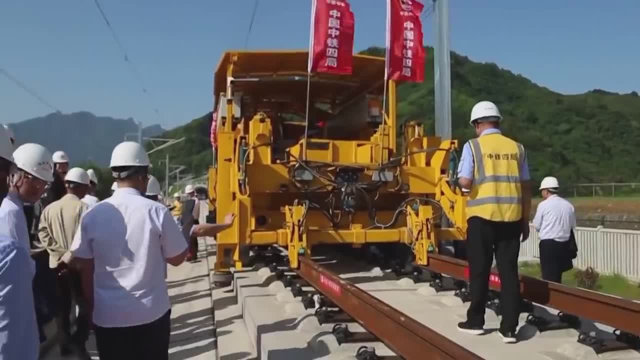 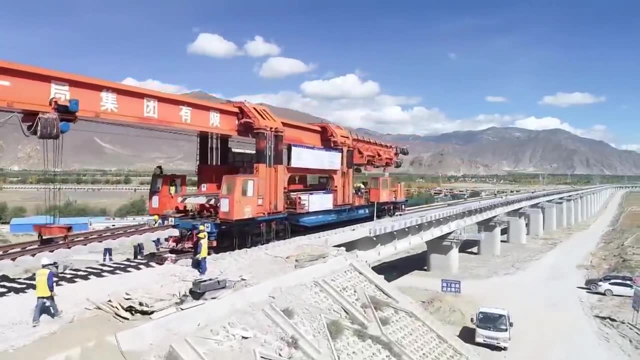 rugged landscapes such as mountains and rivers. It has already contributed towards several high-speed rail projects, including a new link between Inner Mongolia and the rest of the country. Now, if you thought the Iron Monster was giant, wait till you see the Kunlun. 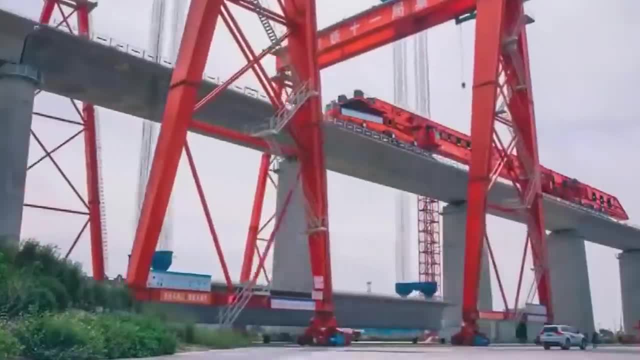 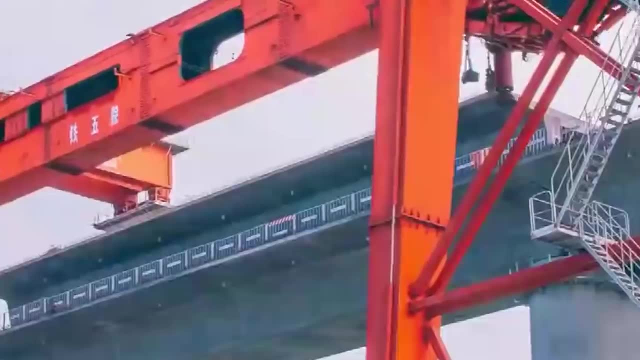 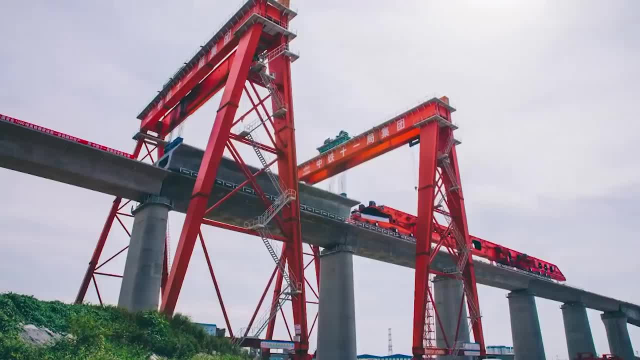 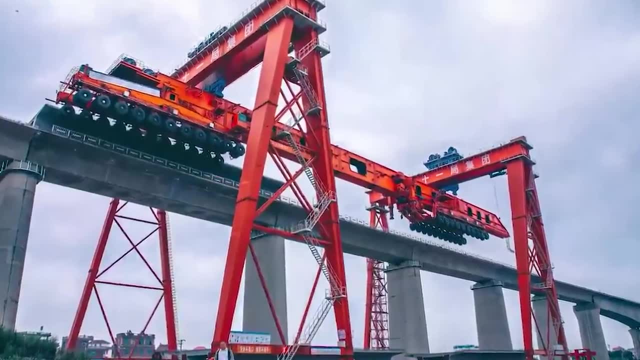 It can also be used as a bridge for construction. It can also be used as a bridge for construction. According to the China Railway Construction Corporation, Kunlun is one of its kind in the world, and it symbolizes a technological breakthrough in the world of road and 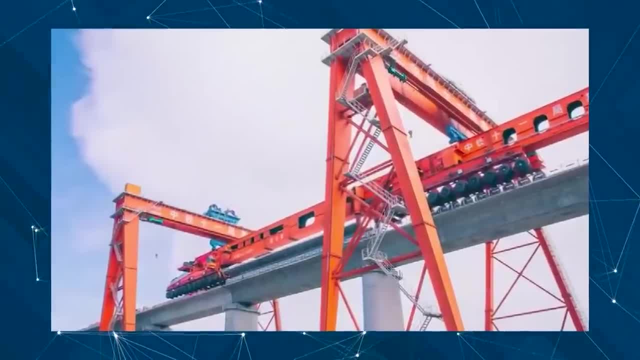 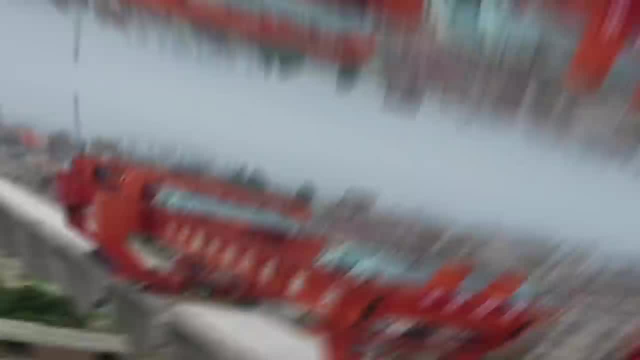 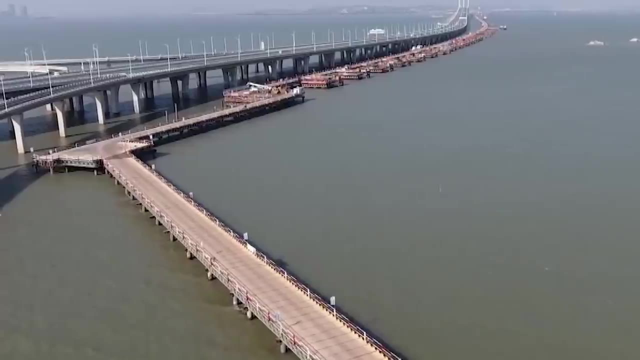 railway bridge engineering. It can also perform the task of intelligence coordination during construction and can solve bridge erection and power supply problems in difficult terrains. In June 2020, Kunlun successfully erected the first 1,000-ton box girder of the Fujian-Zhaimen high-speed railway bridge, The Fujian Bridge. 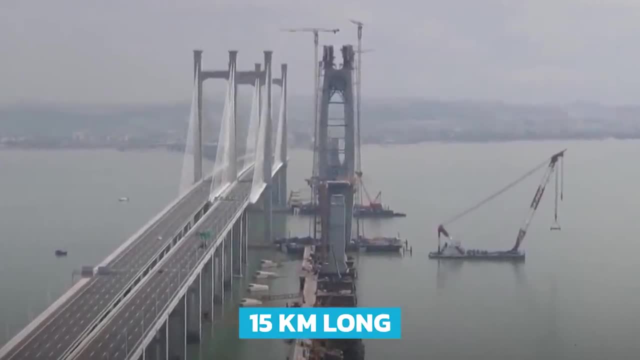 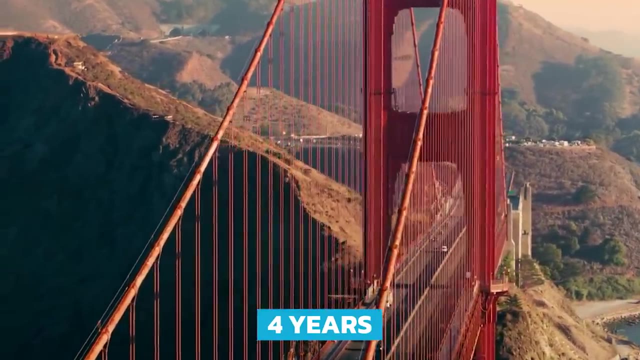 is a cross-sea bridge that is almost 15 km long and is expected to be completed by 2022.. For comparison, it took four years to build the Golden Gate Bridge, which is roughly 3 km long. The Fujian Bridge is almost five times longer than the Golden Gate Bridge. 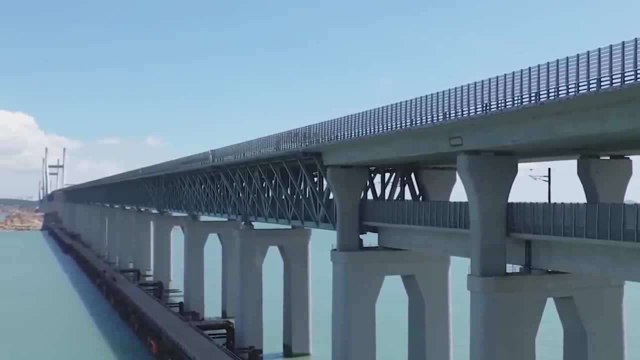 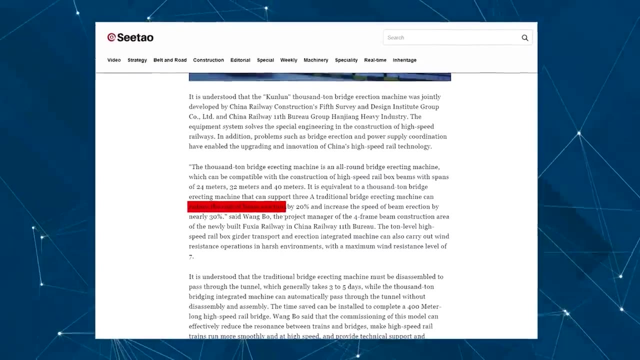 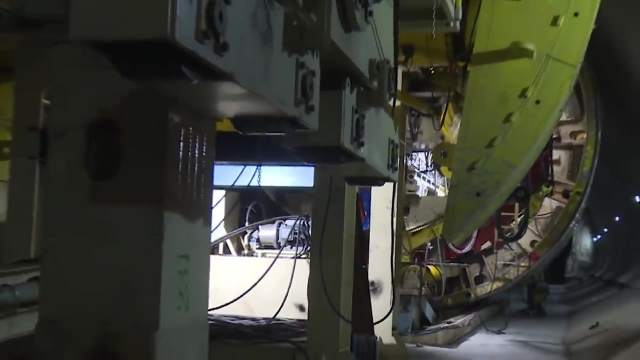 and is expected to be completed in half the duration it took for the Golden Gate Bridge. According to a statement issued by the State Council, Kunlun can reduce about 20% of girder erection costs and speed up the process by 25%. What sets Kunlun apart is its ability to operate. 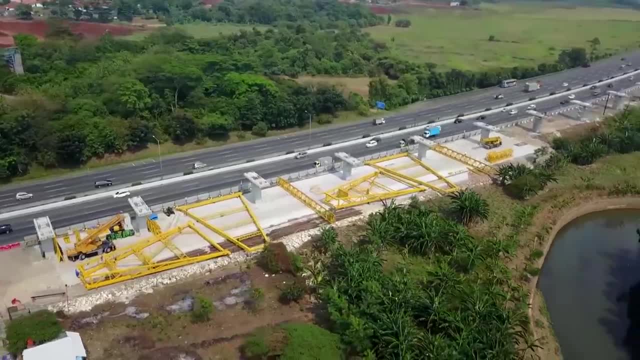 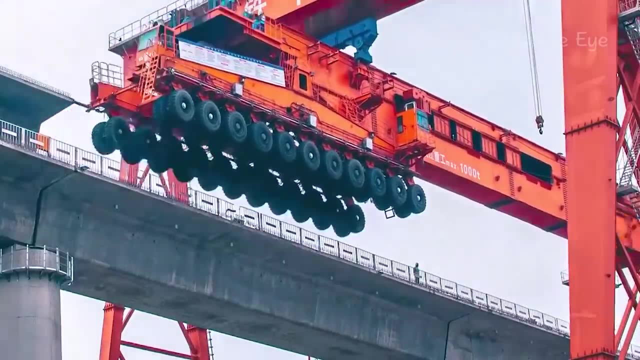 inside tunnels, although it will need to be disassembled before it can pass through a tunnel. In the past year, Kunlun has laid down beams in tunnels, both at tunnels' entrances and exits. It has passed the tunneling test and given China a competitive advantage in low-cost rail and. 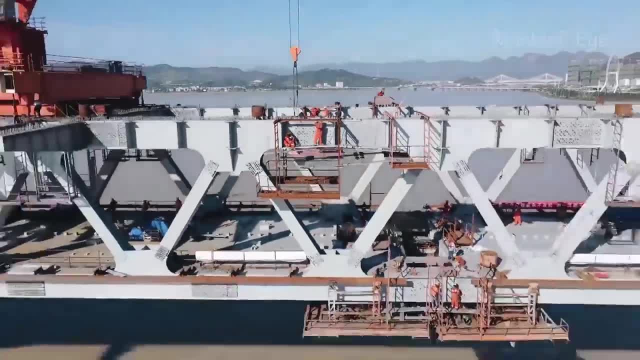 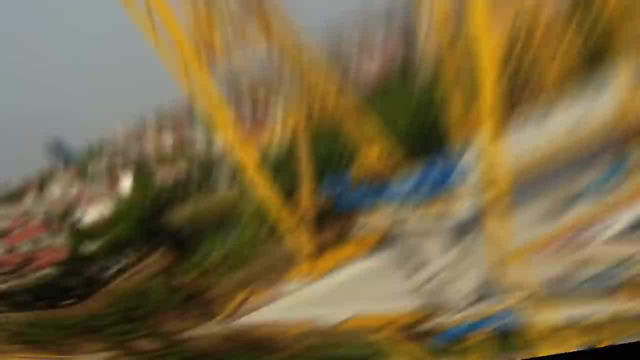 road-based rail Kunlun can be particularly effective in the western region of China, where there are lots of tunnels and deep valleys leading to bridge and tunnel conversions. Kunlun also uses high-strength steel plates that are aviation and submarine grade-level materials. 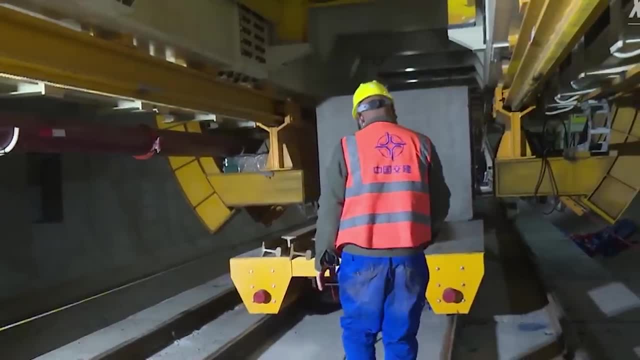 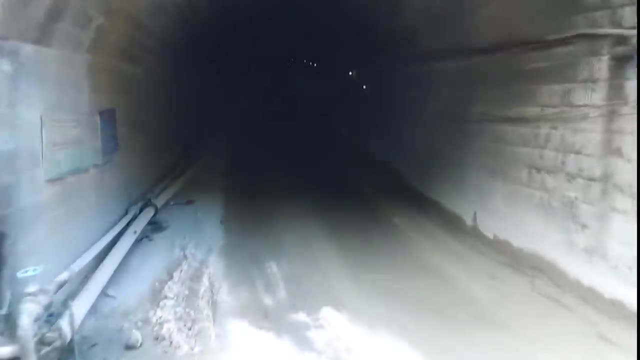 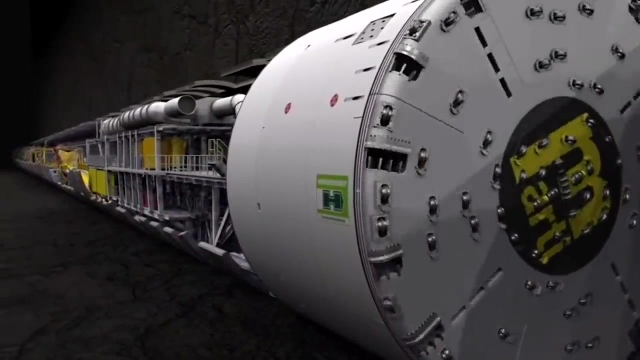 Kunlun also has a laser matrix system that enables it to drive automatically in tunnels by scanning the surrounding environment. It is a pretty handy machine, to say the least. If Kunlun can lay down beams in tunnels, it can only mean that China has finally cracked the code for making big tunneling machines. 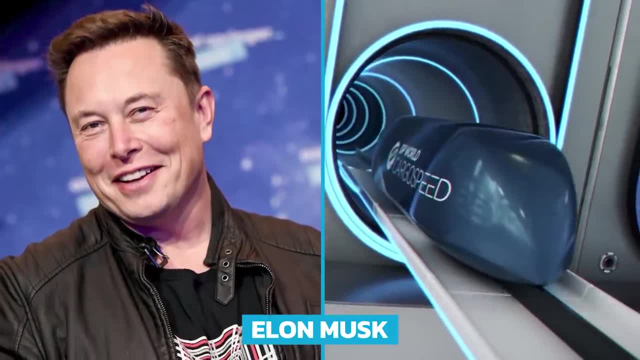 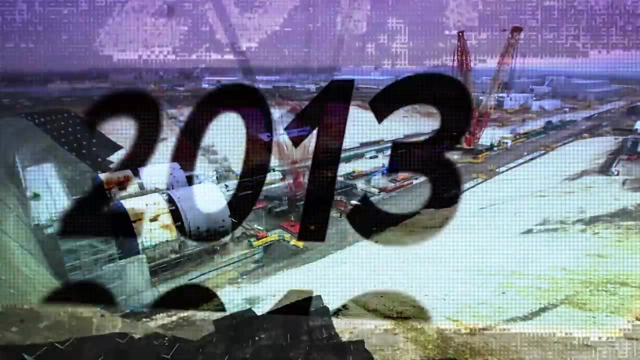 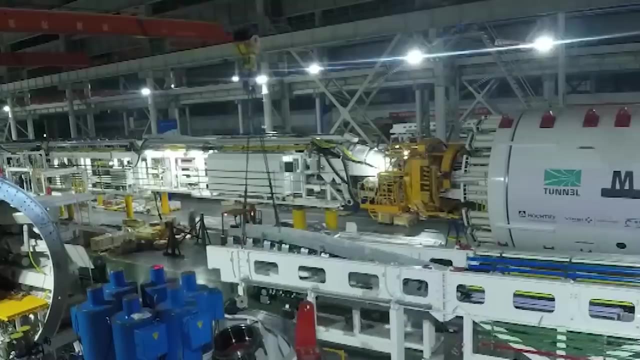 Although the word tunneling these days brings Elon Musk's boring tunnels to mind, China is not too far behind when it comes to boring tunnels. Less than a decade ago, European manufacturers ruled the tunneling machine market and China, like other countries, had to buy tunneling machines from Europe. 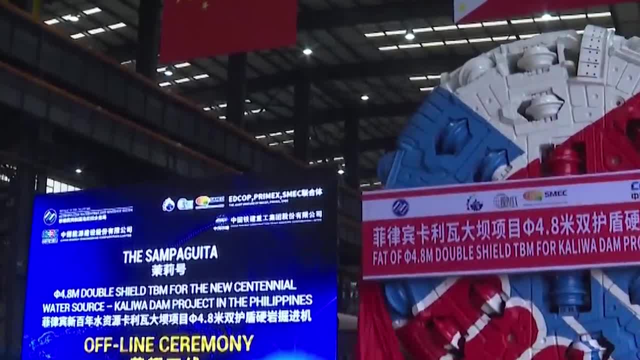 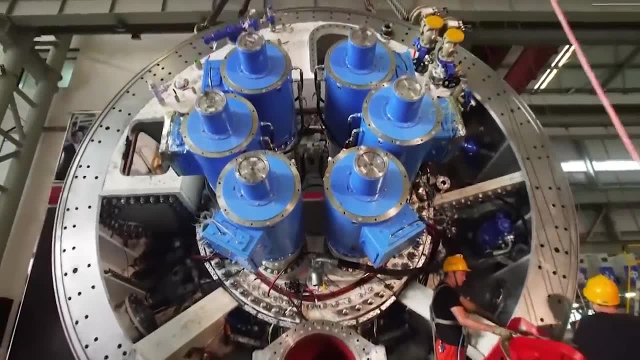 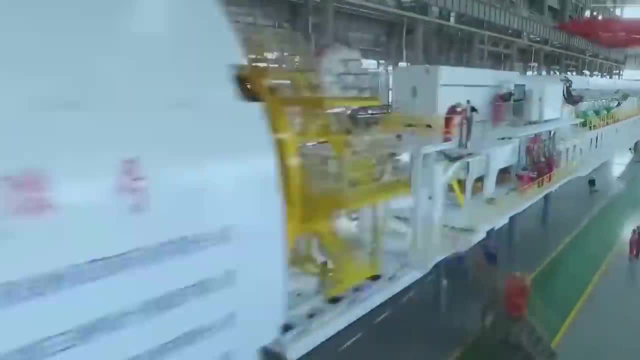 In 2019,, however, China started exporting tunneling machines to Europe For a high-speed railway project between Milan and Verona. Over the last few years, Chinese engineering companies have reverse-engineered tunneling machines and managed to make them in a more efficient and cost-effective manner. as compared to their competitors in Japan and Europe, Chinese tunneling machines can dig up to 10 kilometers of tunnels in a day at a cost of $10 million per tunnel. Compare this to the cost of tunneling in the USA, where each kilometer costs around $50 million. 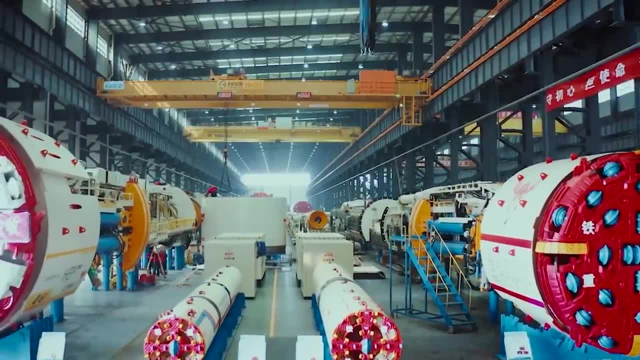 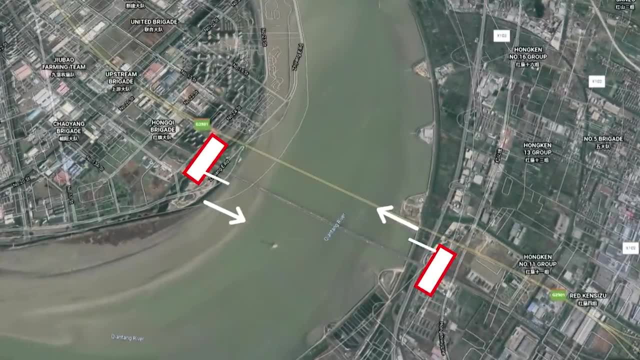 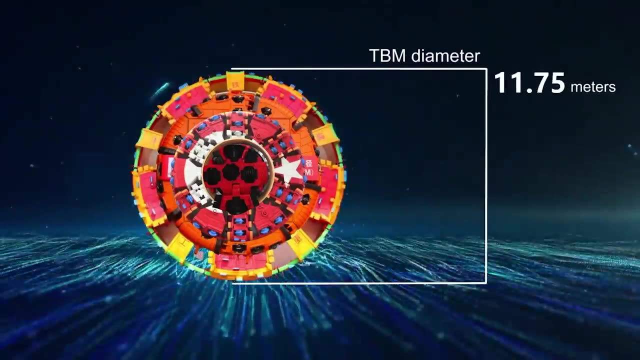 The CRCHI tunneling machine has been domestically built and has been used to tunnel one of the twin tubes in the Genshan East Road Highway, crossing under the Chantang River, in the city of Hangzhou, near Shanghai in China. The CRCHI tunnel building machine has a diameter of 15 meters. 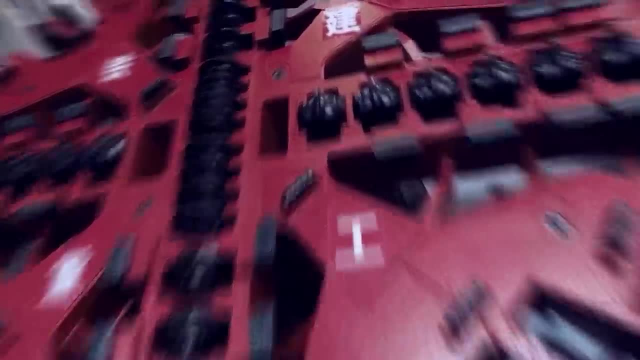 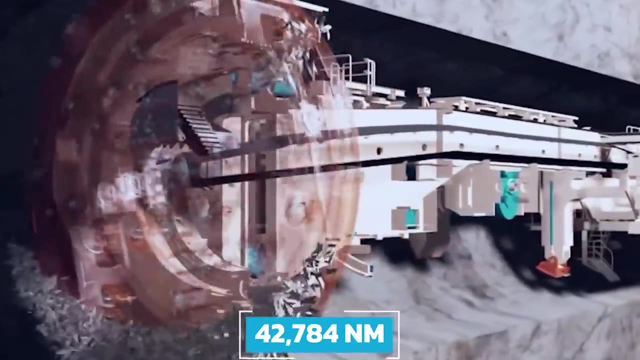 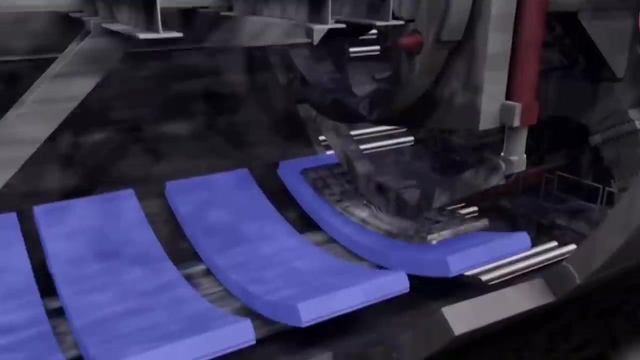 which includes it among the widest tunneling machines in the world. It has an installed power of about 9,755 kilowatts, rated torque of 42,784 Nm and a maximum excavation speed of 50 mm per minute. Like all tunneling machines, it can tunnel and lay down tunneling walls as it plows through. 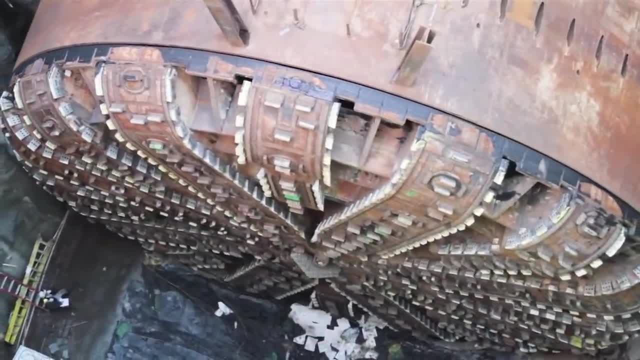 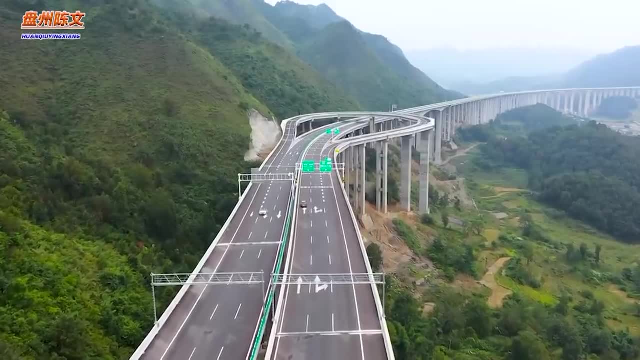 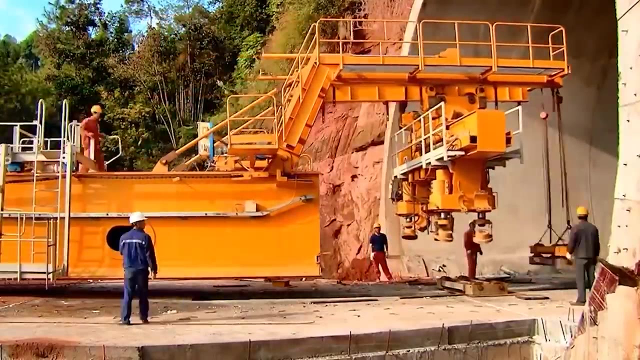 As if this wasn't enough, China is considering mega tunneling machines. The tunneling machines Kunlun and SLJ-900 combined together have given China a very decisive competitive edge when it comes to building road and railway networks. These mega machines form an integrated unit and can lay down tracks for high-speed railway. 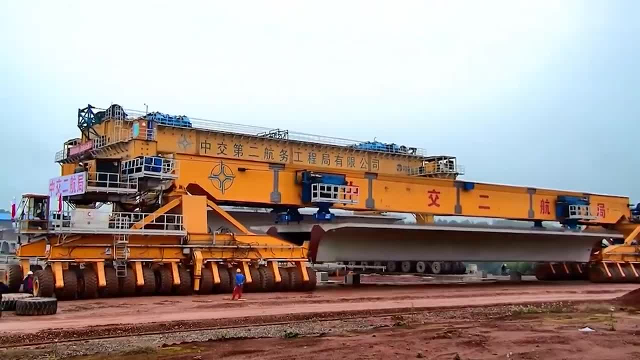 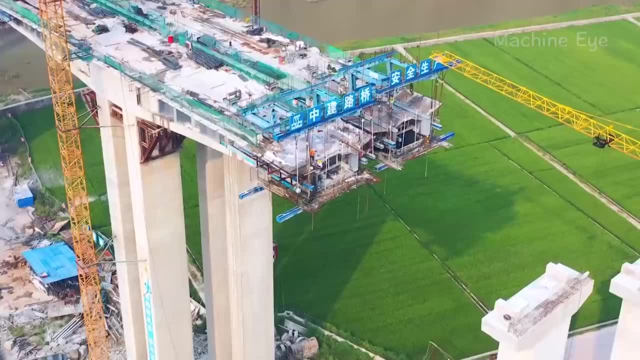 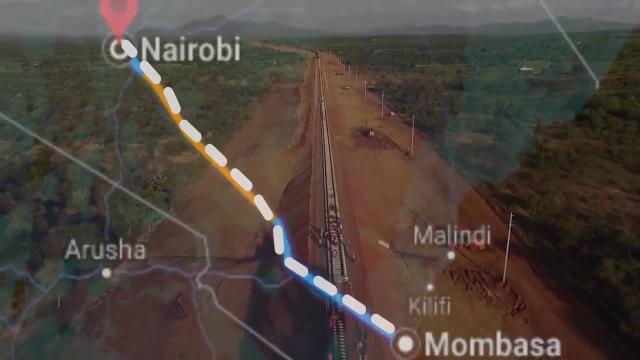 projects and roads over difficult terrains. These mega machines have allowed China to speed up the One Belt, One Road initiative, under which roads and railway networks are being laid down all over the region and not just in China. For instance, China built the Mombasa to Nairobi railway track and completed it 18 months ahead. 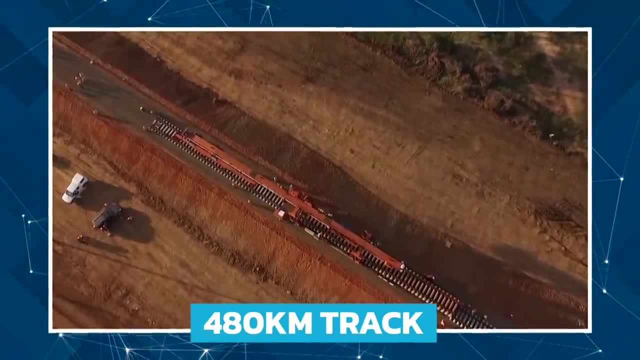 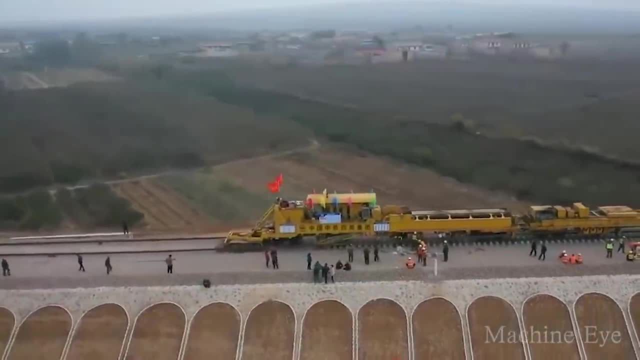 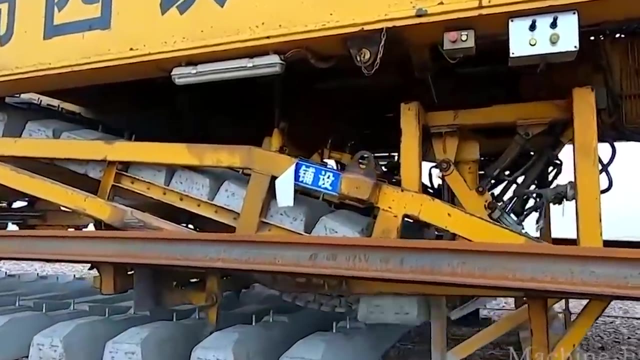 of its time in 2017.. The 480-kilometer track was built at the pace of 700 meters per day. This was done with the help of a track-laying machine that transports prefabricated tracks along the railway line, setting down each track and then rolling on a new track over. 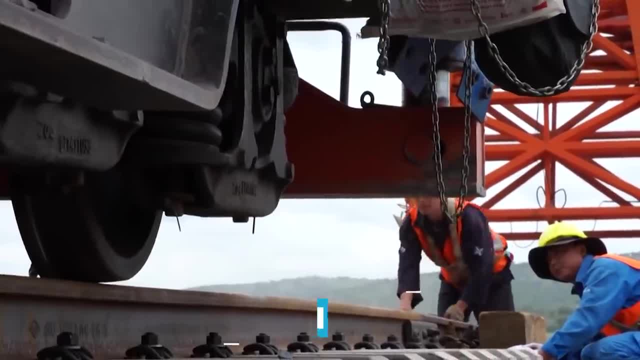 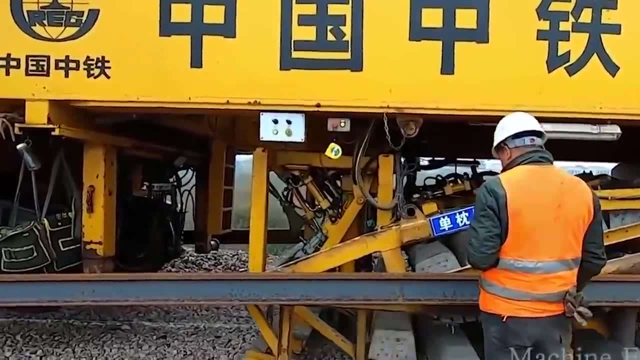 it. Each section of the track can be installed in just 4 minutes. But wait, if you think this is fast, then hold on, because China has developed an even faster track-laying machine. The CYP-500 is a rapid track-laying machine that can lay down 2 kilometers of track in. 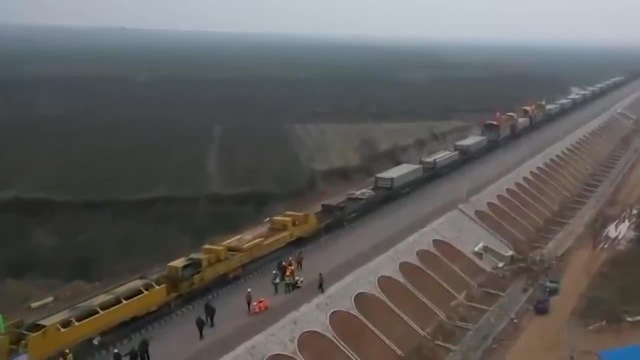 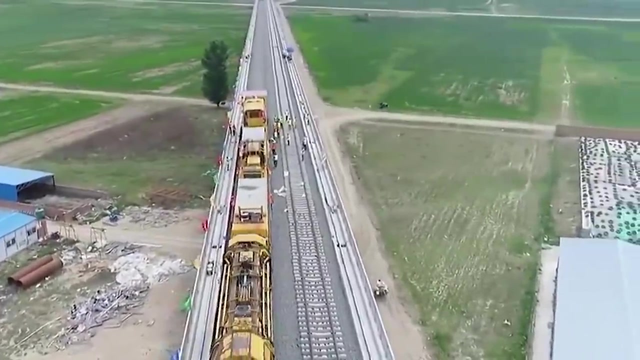 a day In March 2020, the CYP-500 was used to lay down the first section of the China-Laos railway track, which is said to be the longest railway track outside China in Asia, And it is all set to open later this year. 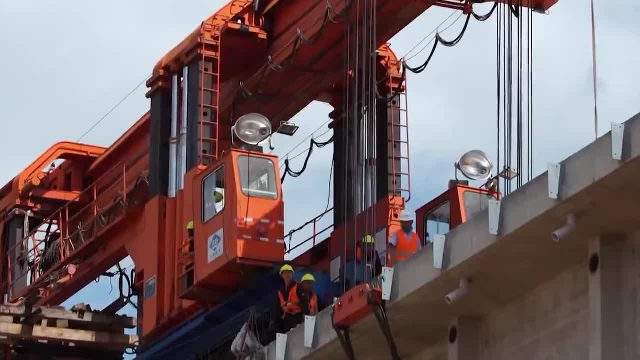 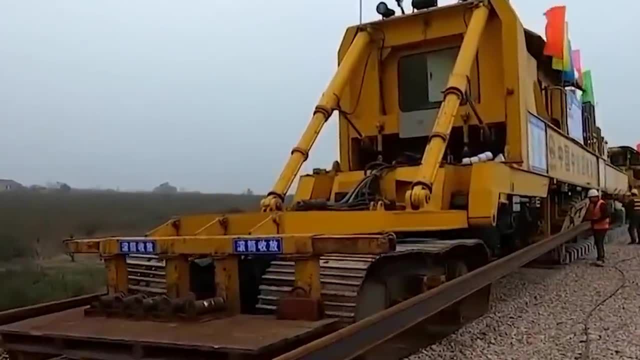 If you compare the railway track China built in Kenya with the one connecting it with Laos, in a span of roughly 4 years, China has gone from laying down 700 meters of track per day to 2 kilometers of tracks per day. Moving away from industrialization, China has also been able to build a new railway track. 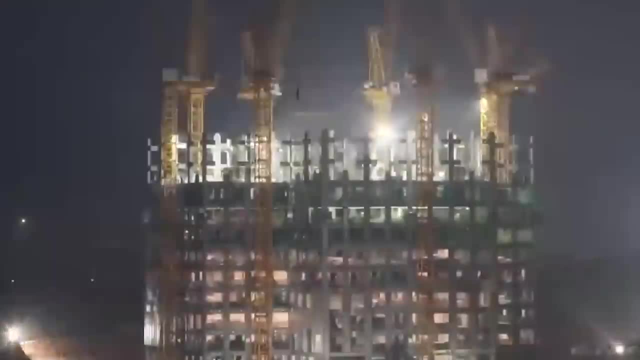 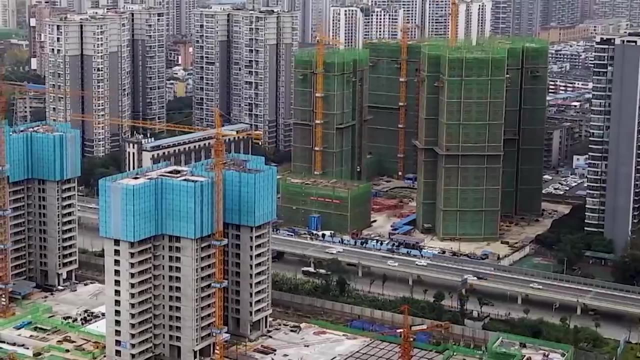 Moving away from industrial-level construction. let's now take a look at how fast China can build in its city centers. Each year, China builds almost half of the world's skyscrapers. But how can China build so many skyscrapers? Well, if you have attentively watched this video so far, then you will already know the. 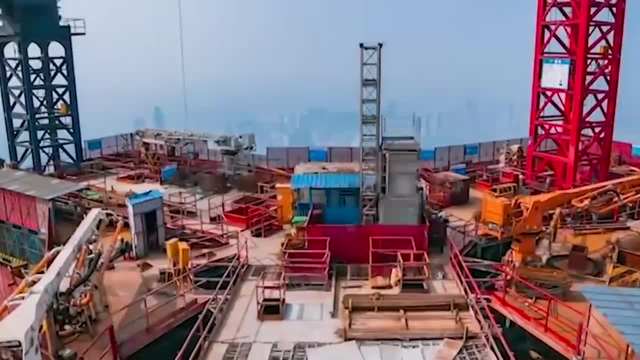 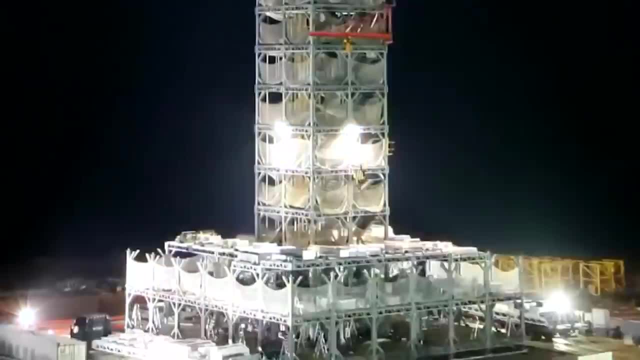 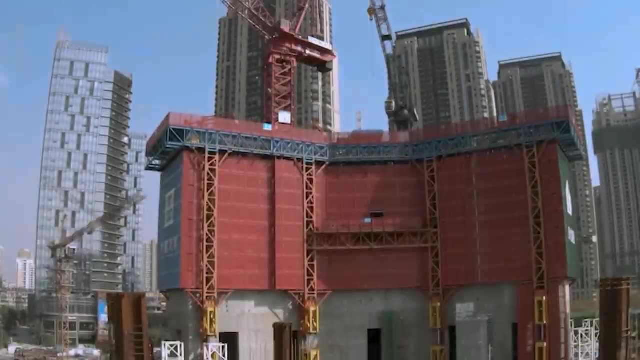 answer: Yes. China has a humongous skyscraper-building machine that weighs a stupendous 2,000 tons. This monstrosity can build an entire floor in 4 days And can remain steady and safe for construction even at a height of 500 meters. 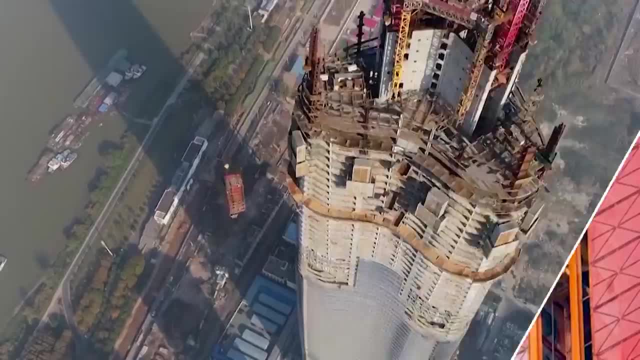 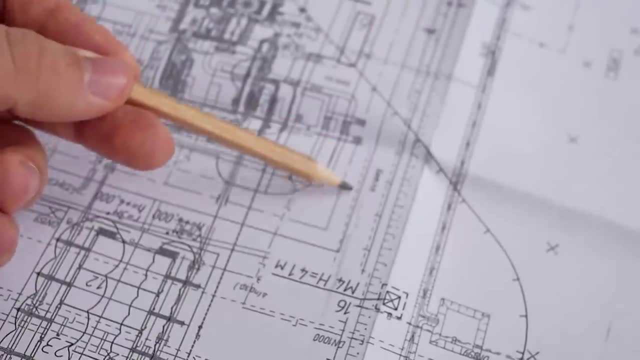 Its weight allows it to easily bear hurricane-force winds. According to Chinese engineers, the wall-climbing monster can increase building speed by over 20%. It was developed over a period of almost three years by designers from the Institute of Engineering Technology in China. 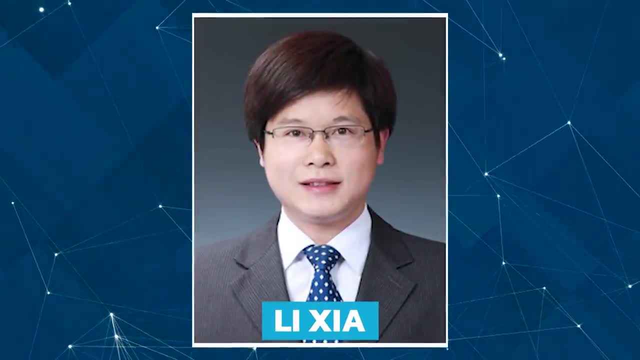 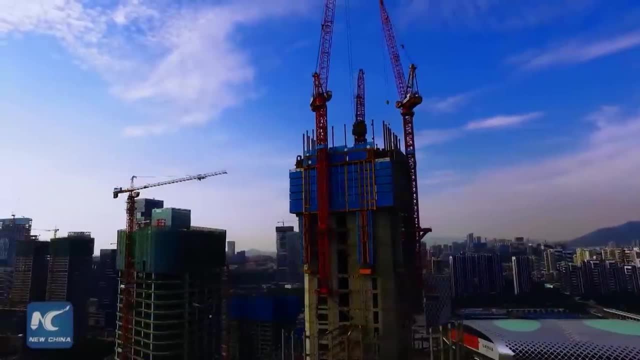 Lai Zhai. one of the mechanical engineers heavily involved in the project, has named the machine Bonot. The Bonot is over 40 meters high and weighs almost 2,000 tons. The development team for the Bonot have obtained eight patents and published five papers on. 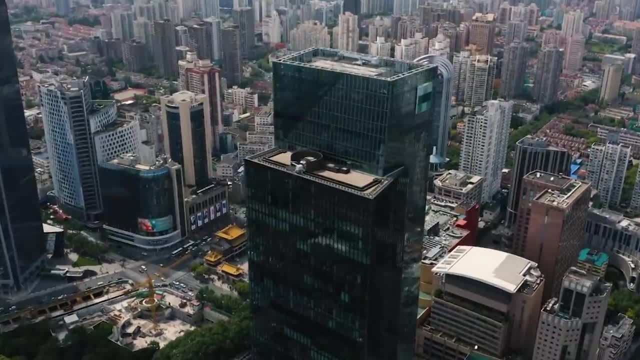 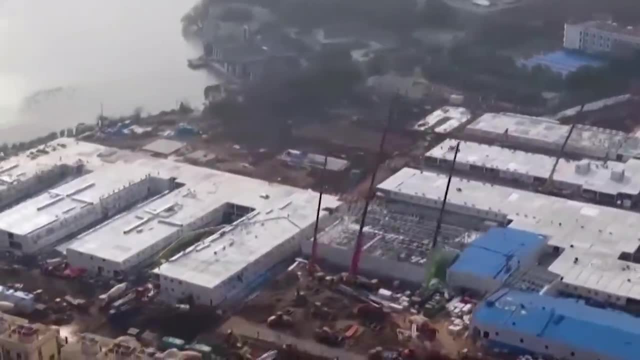 the technologies that have been used to construct it. It's no secret that these technologies have allowed China to build at a rapid rate. We still remember how China managed to build a COVID hospital last year in just six days. They even live-streamed the construction online.